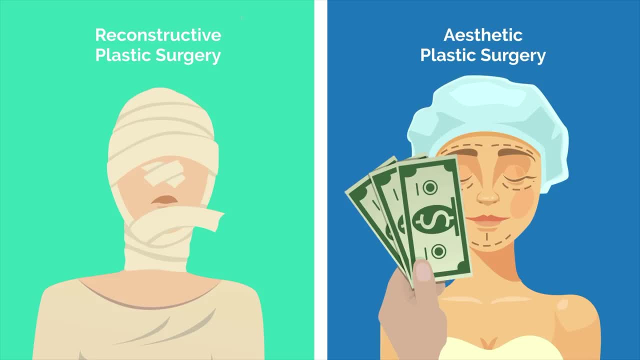 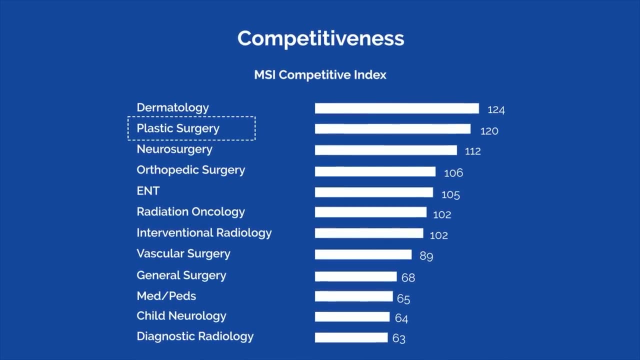 working in aesthetics will, in general, make more than their reconstructive colleagues. That being said, to achieve this compensation, you will first have to match into plastic surgery, which is no easy feat. It is currently ranked number 2 on the MSI Competitiveness Index, neck and neck. 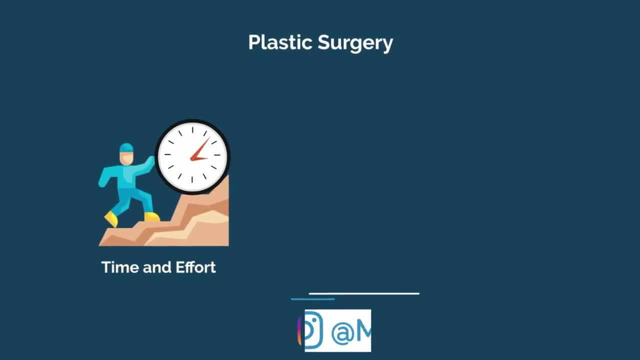 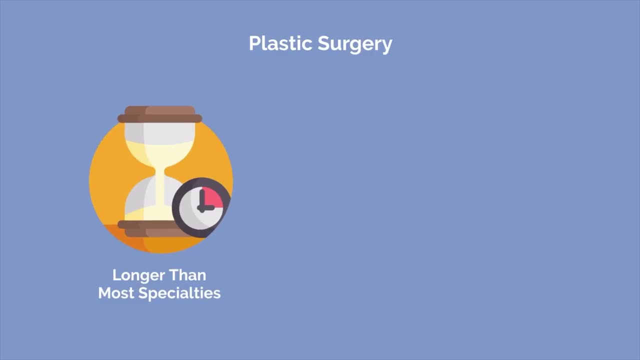 with dermatology in first. You will have to commit a great deal of time and effort during medical school to be competitive for plastics, and even then there is no guarantee that you will match. The training to become a plastic surgeon is also longer than most specialties, at 6-8 years. 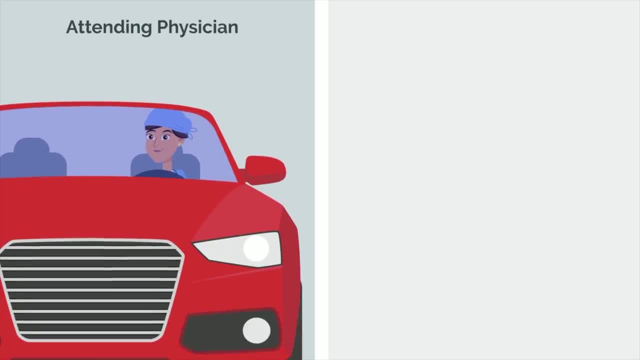 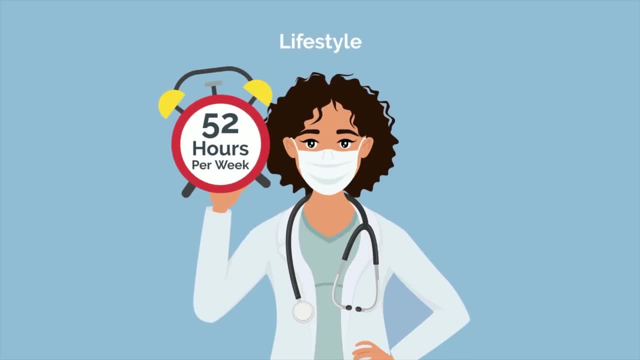 depending on the pathway you take. So, while many of your peers during medical school are already receiving and attending salary, you will still be completing your training Once you begin practicing as a plastic surgeon. however, the least you can do is to become a plastic surgeon. 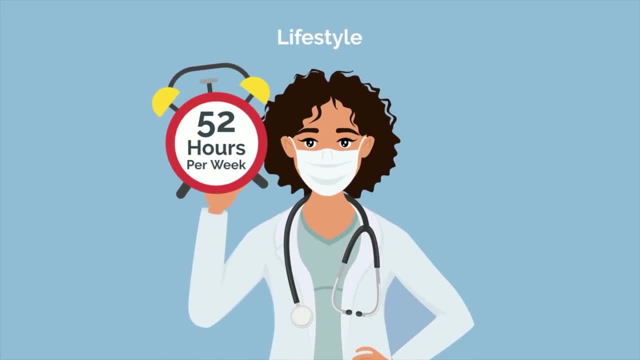 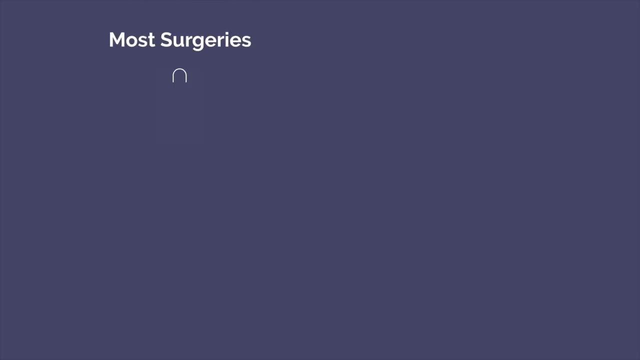 The lifestyle is often pretty good. Plastic surgeons work an average of 52 hours per week, which is less than many of the other surgical specialties, but middle of the pack when looking at all specialties. Most surgeries are also non-urgent, so call typically isn't terrible. 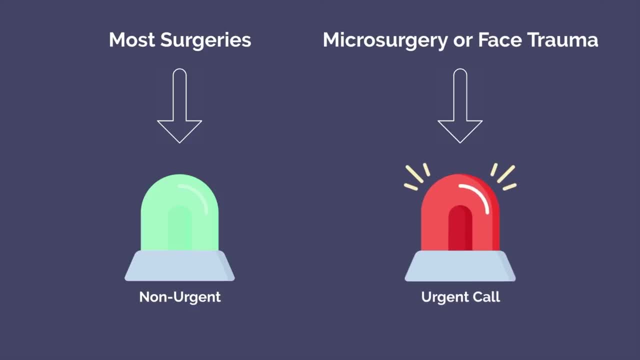 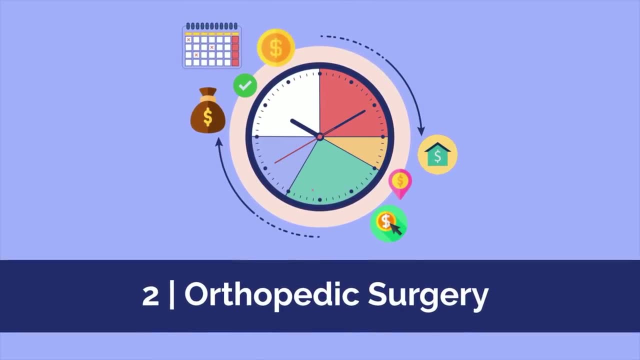 Keep in mind, though, that if you choose to do microsurgery or handle face trauma, your call obligations can be more taxing. Number 2 is orthopedic surgery, which focuses on the surgical management of the musculoskeletal system, including the extremities, spine. 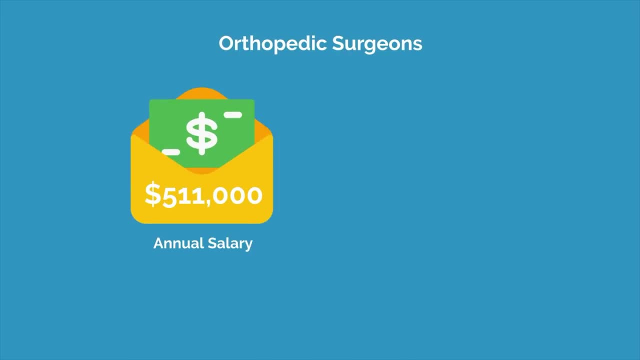 and associated structures. Orthopedic surgeons have an average annual salary of $511,000 and work an average of 57 hours per week, yielding an average hourly wage of $179 per hour. Much like plastic surgery, orthopedic surgery is consistently in the top 3 highest. 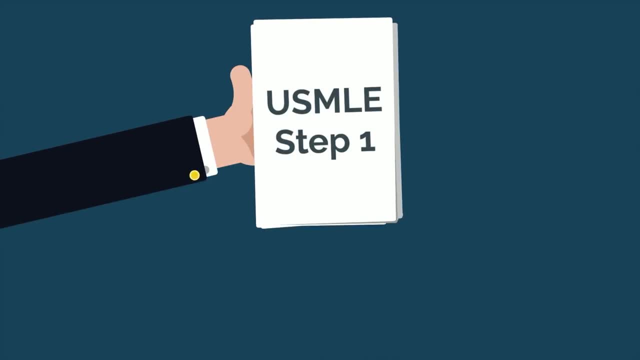 paid specialties, right in the mix with plastics and neurosurgery. Similarly, it is also one of the more competitive specialties to match into, as your USMLE Step 1 score and 1 rep match on bench press will have to exceed 500, which can be a big barrier to entry for prospective applicants. 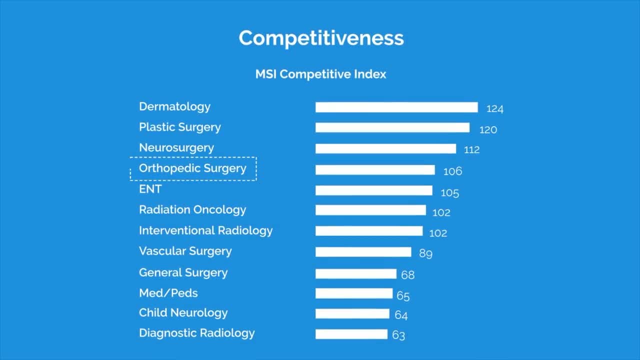 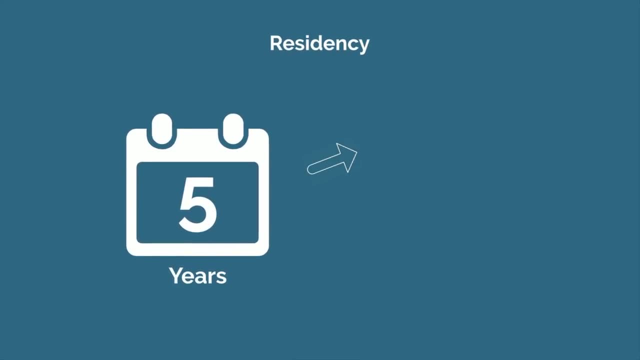 All jokes aside, it is ranked number 4 on the MSI Competitiveness Index, which means more time and effort spent during medical school to make yourself a competitive applicant. Ortho residency is 5 years, which is standard for most surgical specialties. 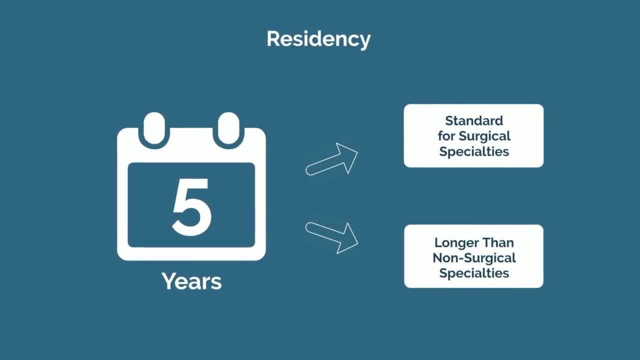 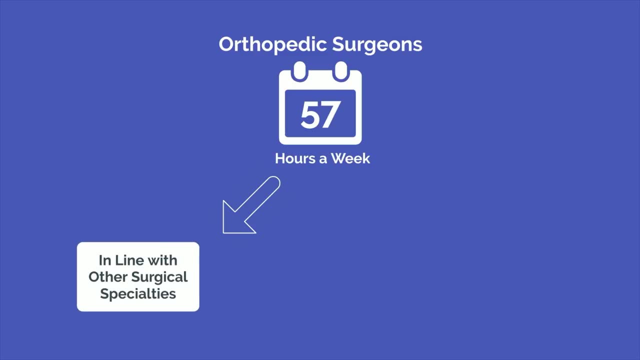 but longer than many non-surgical specialties. Longer residency programs do exist, which include additional research experience. Orthopedic surgeons work an average of 57 hours a week, which is in line with many other surgical specialties, but on the higher end compared. 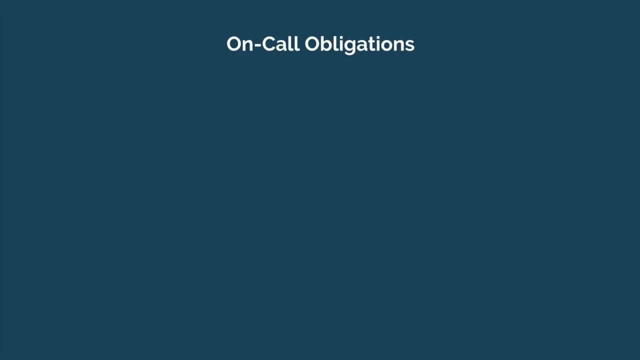 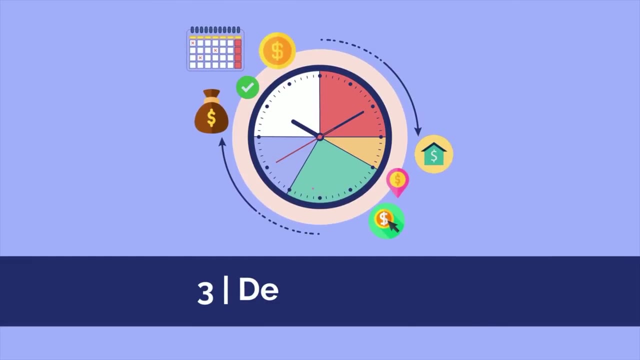 to all specialties. On-call obligations will vary depending on your choice of subspecialty. If you choose to subspecialize in trauma, for instance, be prepared for a heavier call schedule. Number 3 is dermatology, which focuses on the management of diseases involving the skin, hair and nails. Dermatologists. 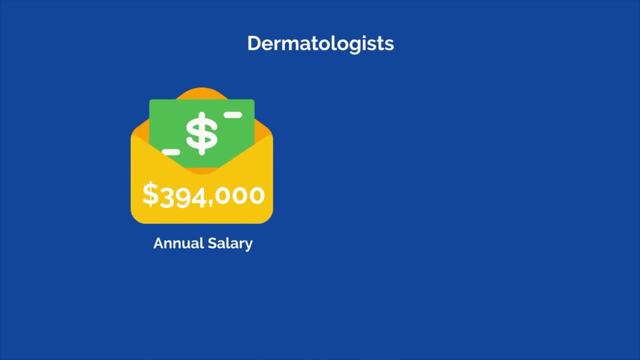 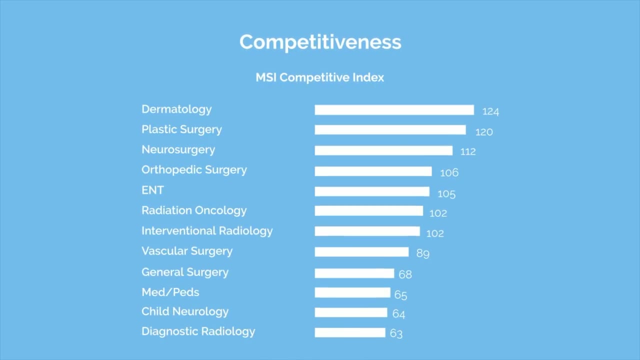 have an average annual salary of $394,000 per year and work an average of 45 hours per week, averaging $175 per hour. Dermatology is currently ranked number 1 on the MSI Competitiveness Index, as it is known to have a great lifestyle and is the only specialty in the top 5, that is. 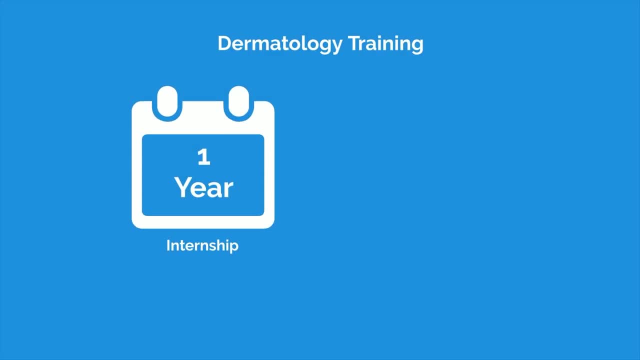 non-surgical. To become a dermatologist, you will have to complete a one-year internship, followed by 3 years of dermatology residency, for a total of 4 years of training after medical school, which puts dermatology in the middle of the pack when it comes to length. 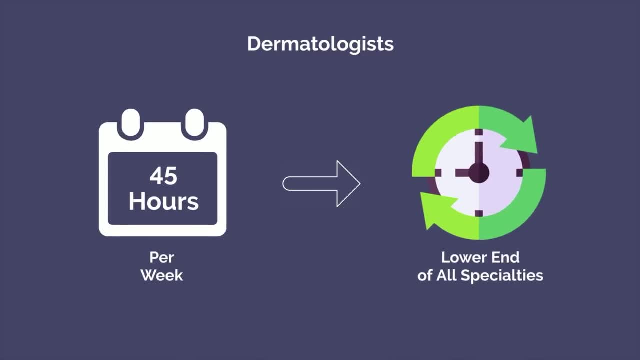 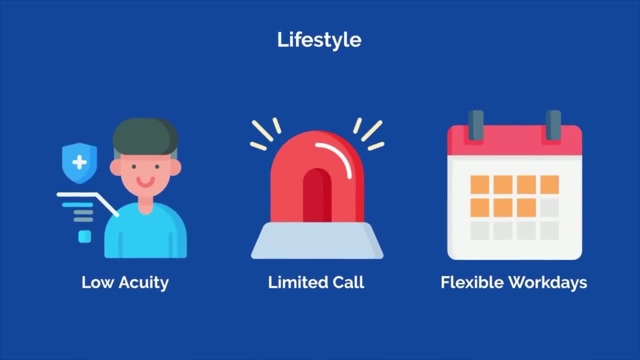 of training, Dermatologists work 45 hours per week, which is toward the lower end of all specialties. Given the outpatient nature, low acuity of medical conditions, limited call and flexible workdays, dermatology is known for having a cush lifestyle relative to other medical specialties. 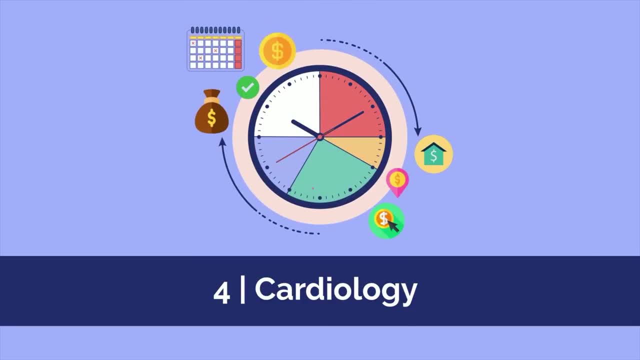 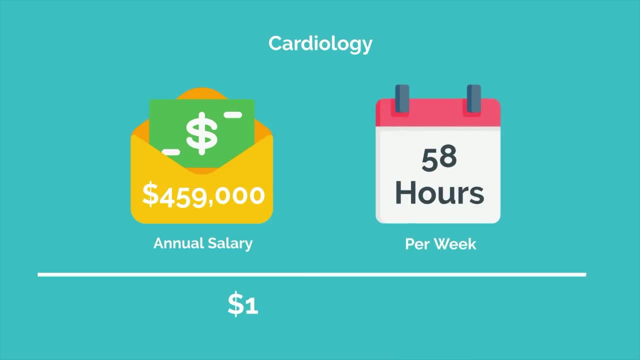 Number 4 is cardiology, which focuses on diseases of the heart and blood vessels. Cardiologists have salary of $459,000 per year and work an average of 58 hours a week, yielding an average hourly wage of $158 per hour. Cardiology is the first specialty on our list that does not have a dedicated 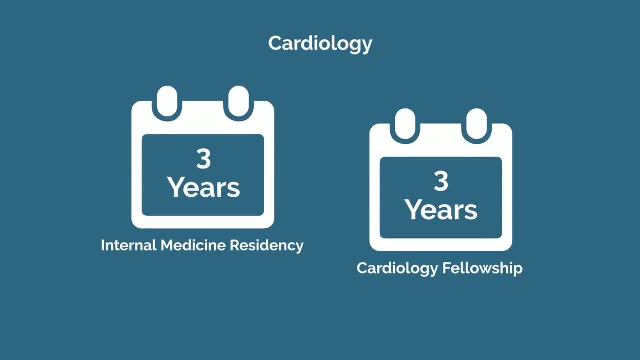 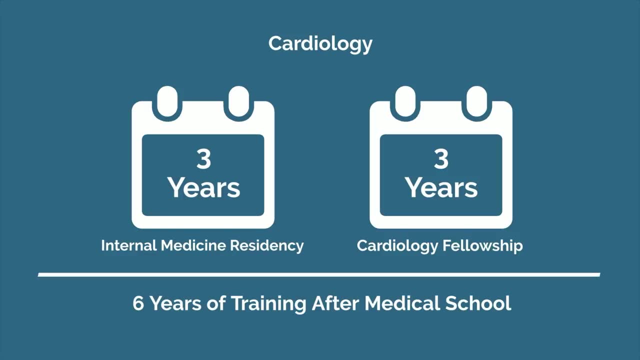 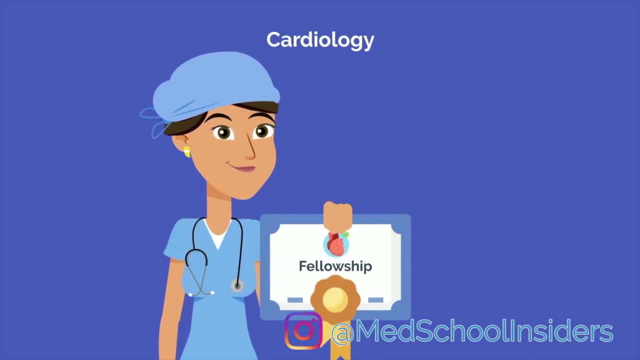 residency. Instead, you must first complete 3 years of internal medicine residency, followed by 3 years of cardiology fellowship, for a total of 6 years of training after medical school. Although it is difficult to compare the competitiveness of cardiology to other specialties on our list, due to the fact that it is a fellowship and not a residency, it should be. 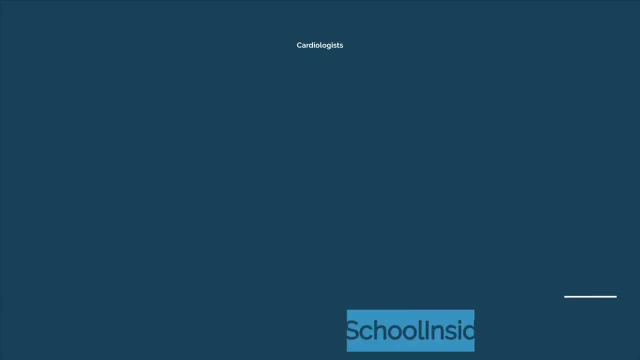 noted that cardiology is one of the most competitive internal medicine fellowships to get into. Cardiologists work an average of 58 hours per week, which is toward the higher end when compared to most other non-surgical specialties. This time is split between clinic cath, lab performing. 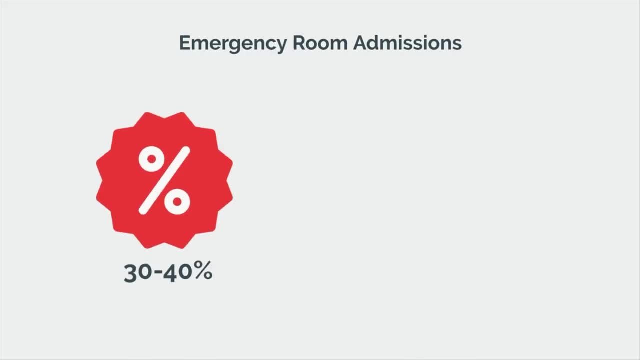 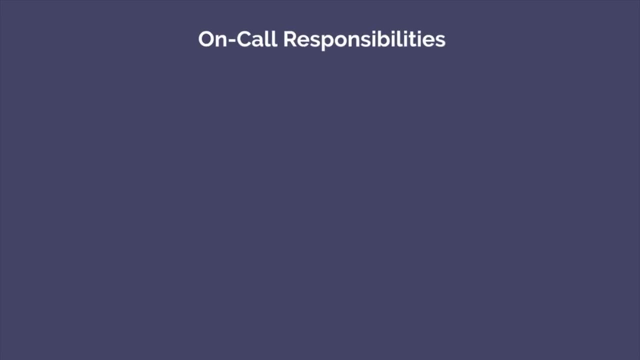 procedures, general rounds and research Of note. 30-40% of emergency admissions are cardiac related, so there is certainly no shortage of work. if you're a cardiologist, On-call responsibilities will vary depending on your subspecialization. If you choose to subspecialize in interventional 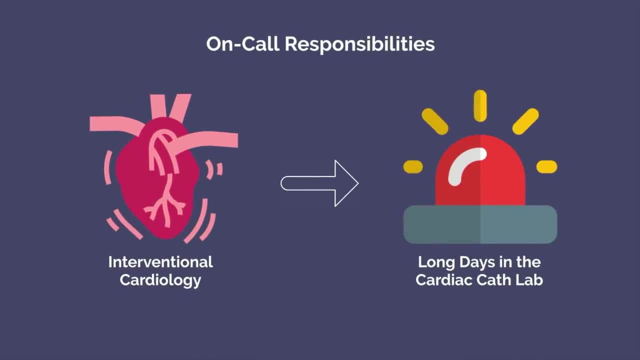 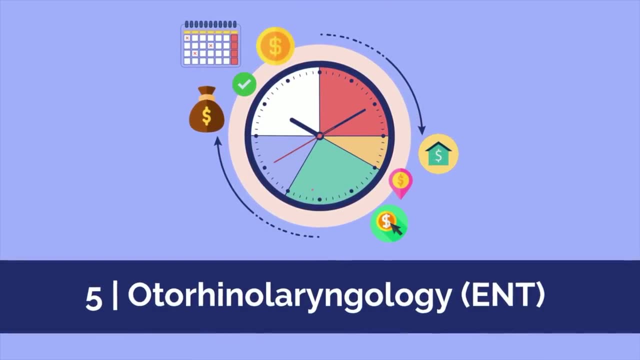 care. for instance, you can expect lots of call with long days in the cardiac cath. lab. Number 5 is otorhinolaryngology, or ear, nose and throat, which focuses on the surgical management of diseases of the head and neck region, Ear, nose and throat. doctors or ENTs. 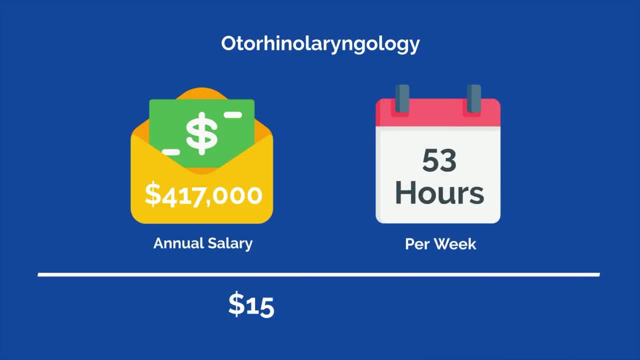 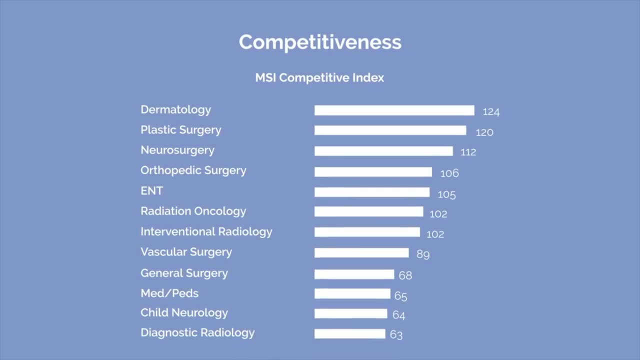 have an average salary of $417,000 per year and work an average of 53 hours per week, averaging $157 per hour. ENT is a highly competitive specialty, consistently ranking number 5 on the MSI Competitiveness Index, right after dermatology, plastic surgery, neurosurgery. and orthopedic surgery. ENT residency is 5 years, which is the standard for most surgical specialties, but longer than many non-surgical specialties. Longer residency programs do exist, which include additional research experience. ENTs will work an average of 53 hours per week. 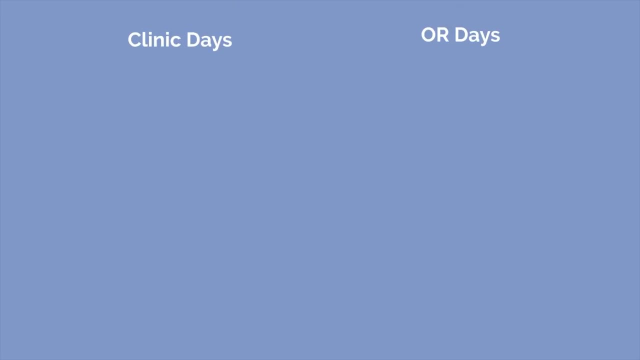 which is middle of the pack when looking at all specialties. Work is typically split between surgery and clinic, with clinic days generally having regular 9-5 hours and OR days being half days or full 12 hour days, depending on complexity of the cases Given the greater proportion of time. 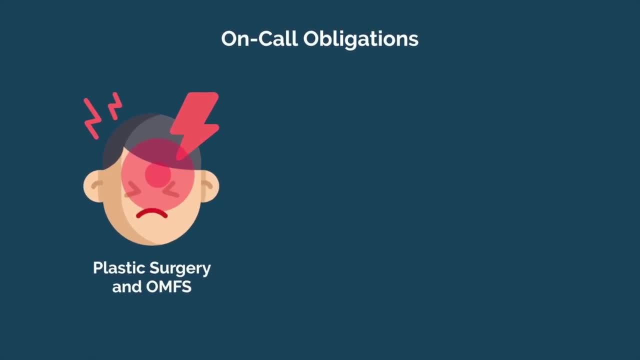 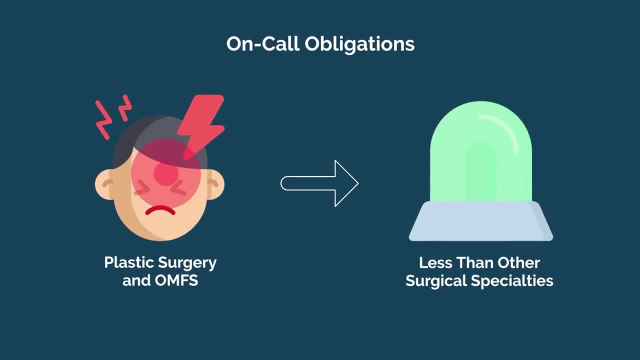 in the clinic, coupled with the fact that ENT typically splits face call with plastics and OMFS, on-call obligations are typically less than other surgical specialties. This can vary, though, depending on the hospital or institution you work for. Number 6 is emergency medicine. 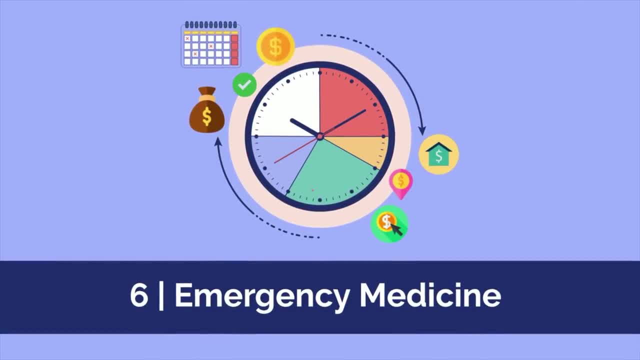 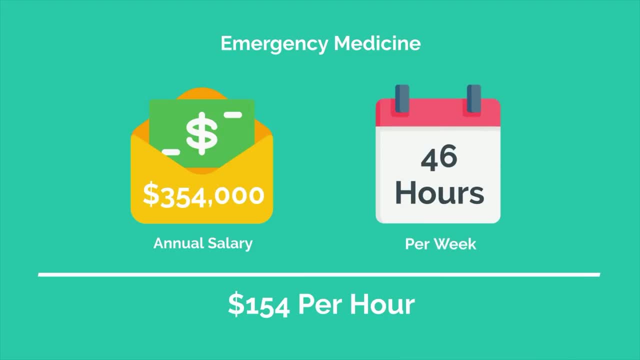 which focuses on the treatment of acutely ill patients with urgent healthcare needs. Emergency medicine physicians have an average salary of $354,000 and work an average of 46 hours per week, averaging out to $154 per hour. In terms of competitiveness, emergency medicine is 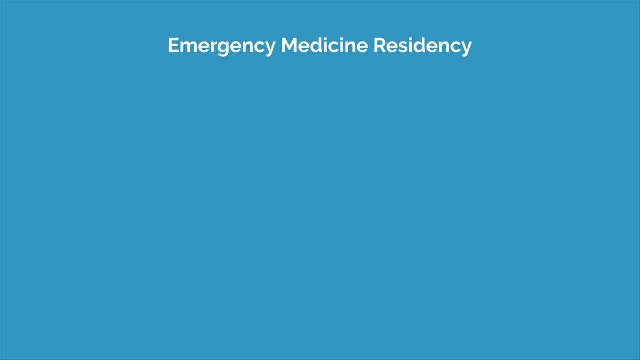 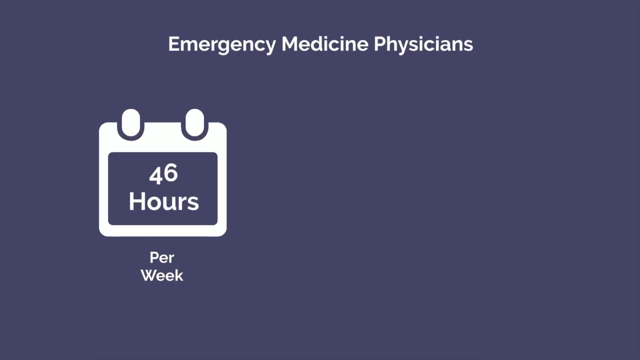 at the lower end of the MSI Competitiveness Index, at number 17.. It is also at the shorter end of residency lengths, at just 3-4 years of training after medical school. Emergency medicine physicians will work on average 46 hours per week, which is towards the lower end. of all specialties. They are also unique in that they do shift work, meaning that they clock in and clock out and don't take work home with them, which is something you can't say about many medical specialties. Emergency medicine is not without its downsides, though, Although many people view. 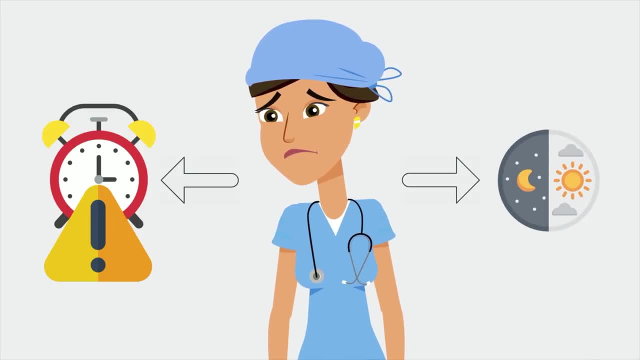 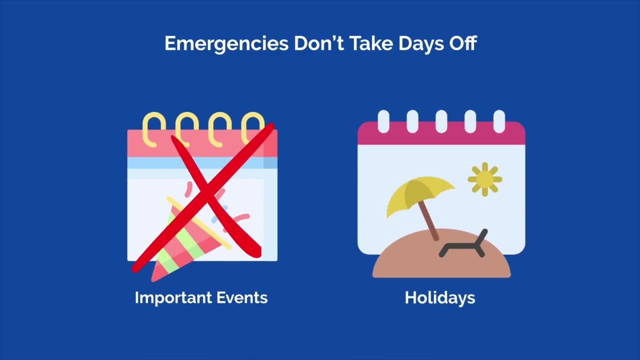 shift work as a positive. it also means that you might end up working irregular hours, so a regular circadian rhythm can be hard to come by Emergencies. don't take days off either, so it is not uncommon to miss important events or holidays, particularly when training or when you. 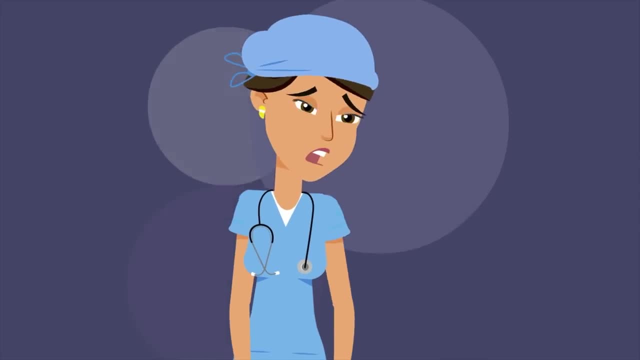 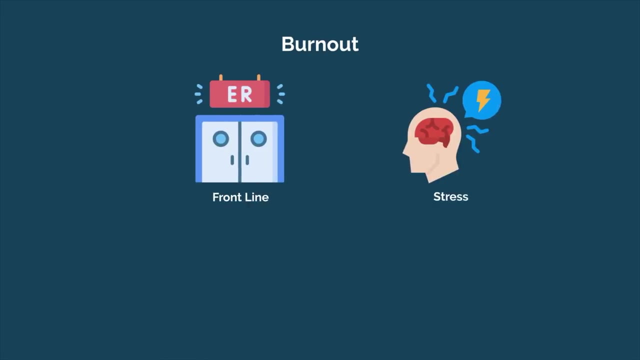 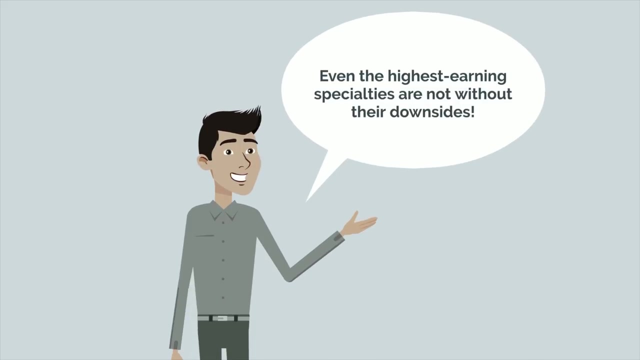 are a freshly minted attending EM. physicians also experience some of the highest rates of burnout, despite working fewer hours than most other medical specialties, which can be attributed to working on the front line: consistent, high intensity and stress, unpredictability, increasing charting demands and irregular circadian rhythm. As you can see, even the highest earning, rates are not the same as the highest earning rates on the other sides. This is why money, although important, should not be the only factor when choosing a specialty. It is much more important to find a specialty that is a good fit and you enjoy doing, If you have your eyes set on.